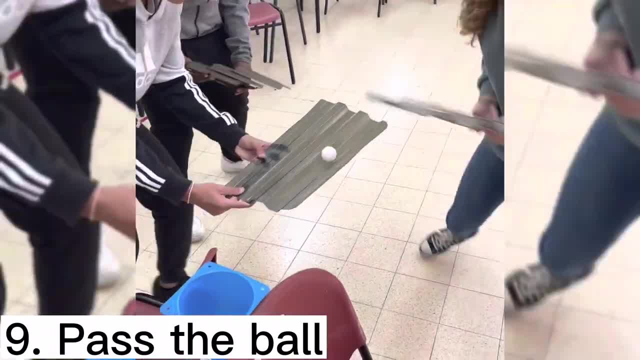 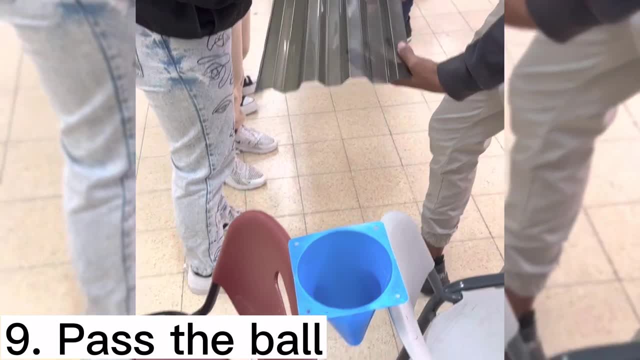 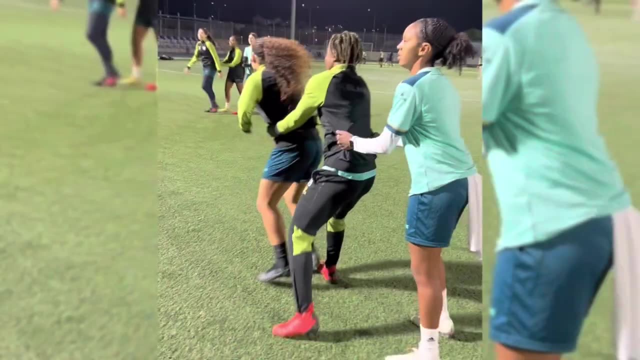 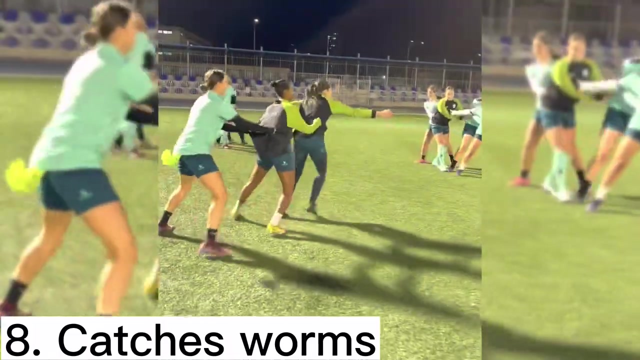 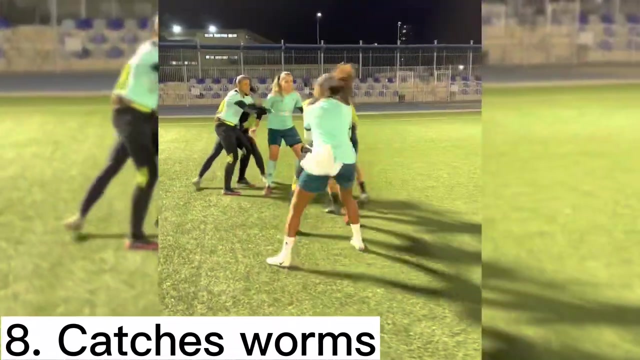 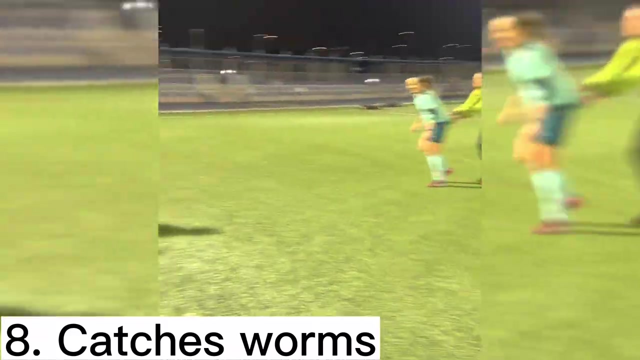 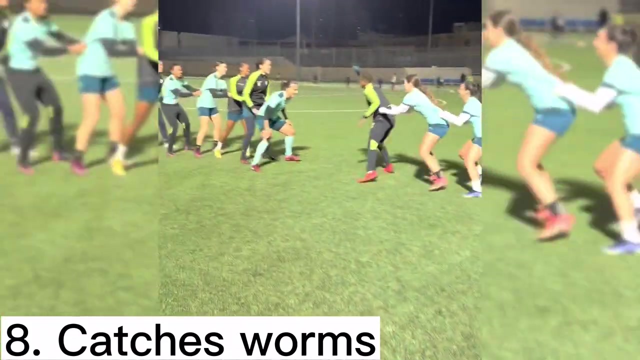 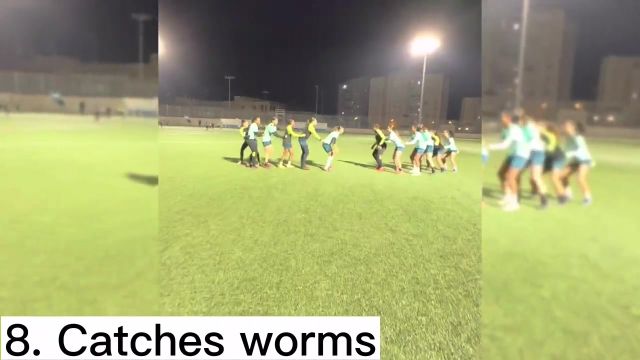 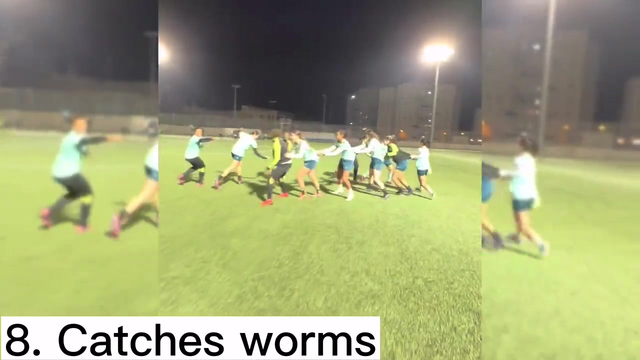 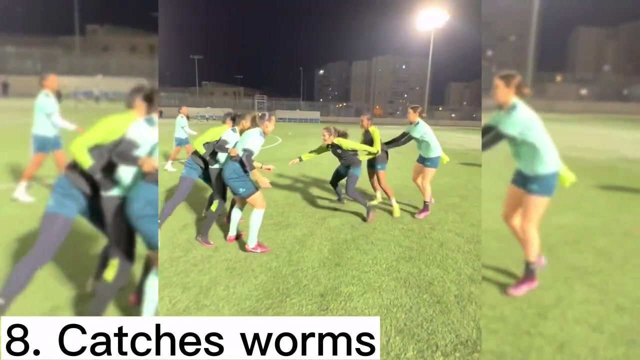 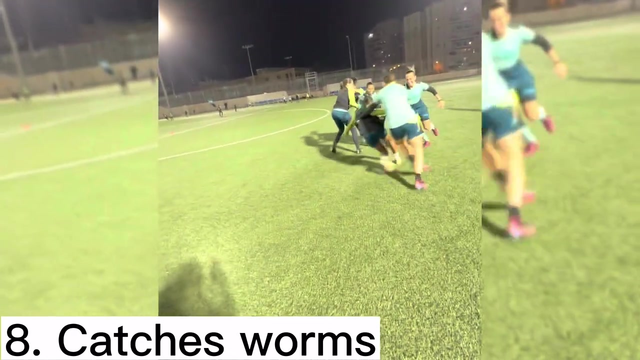 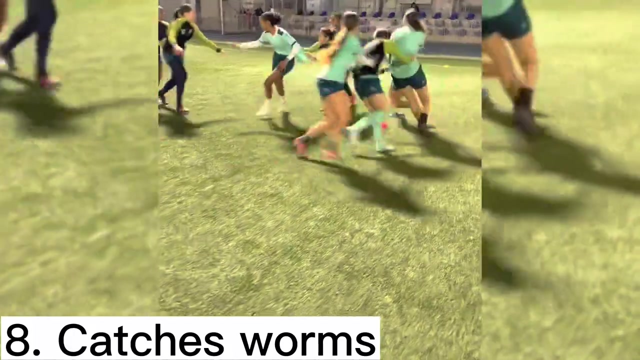 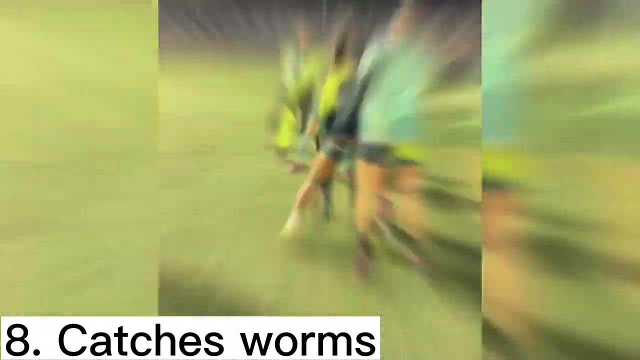 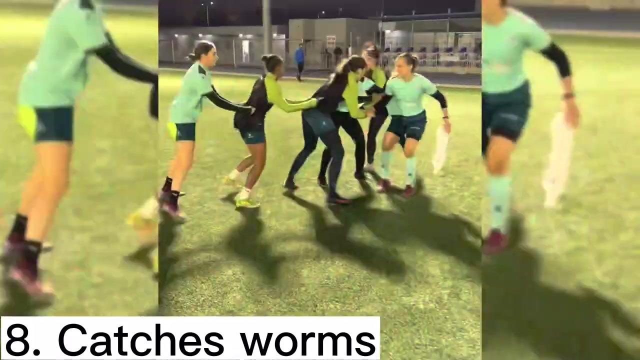 Yaffe, Yaffe, Can I show you In the bazaar with a lot of people Out of nowhere, a man of the people. Look over there. Everyone is doing their best And they are coming Oh. 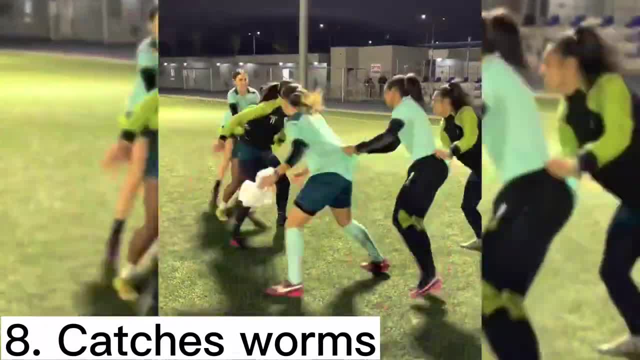 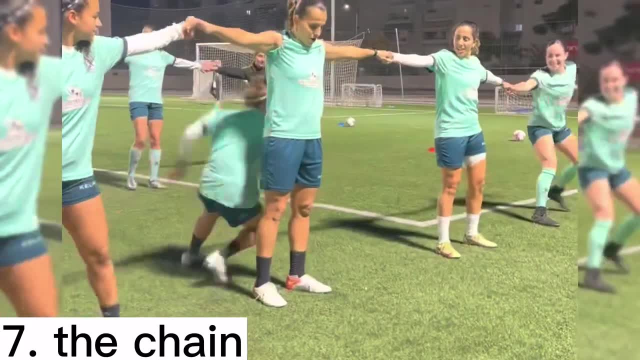 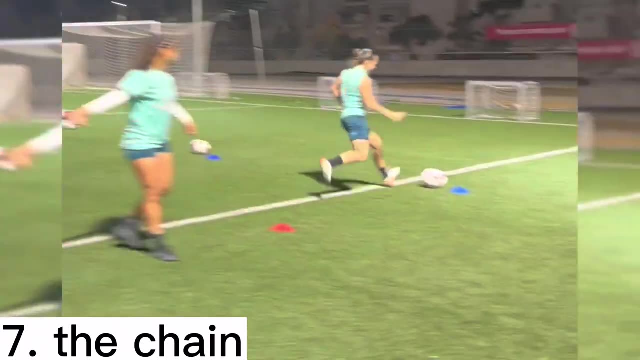 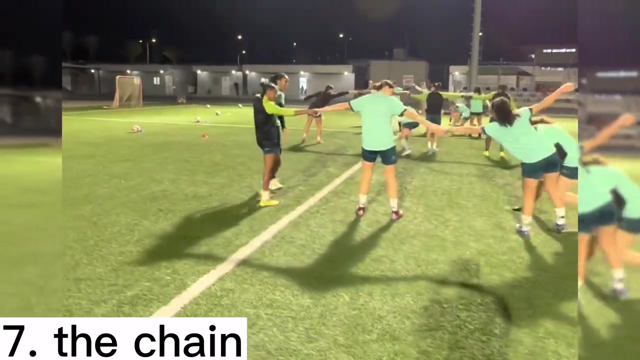 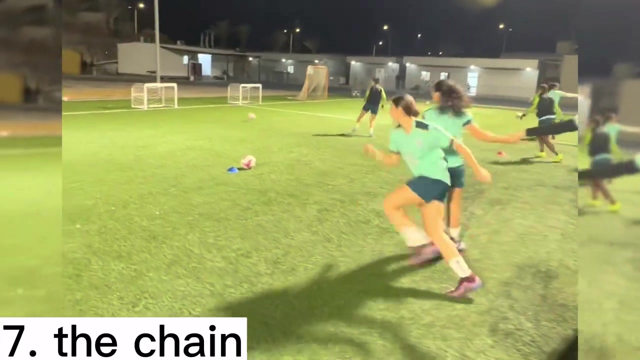 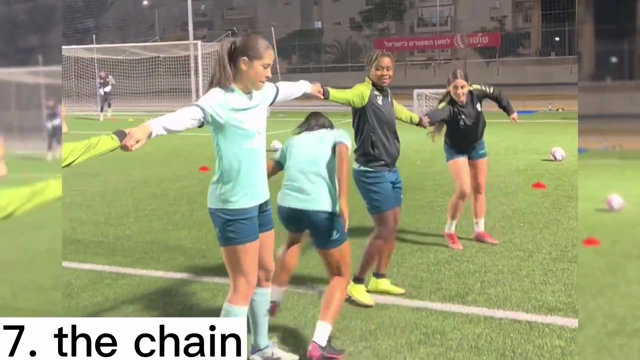 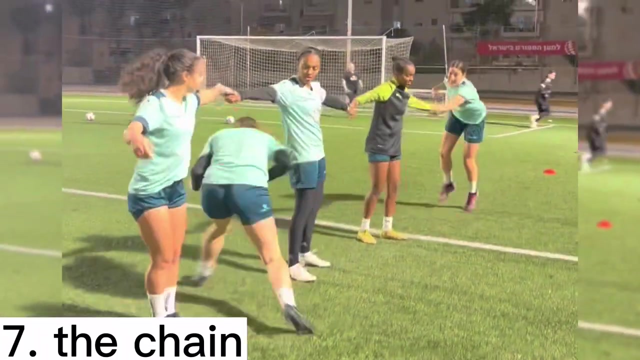 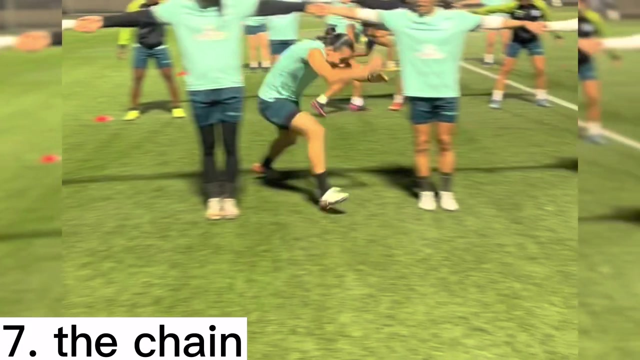 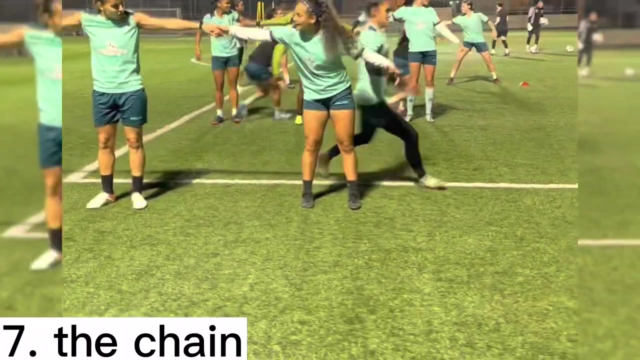 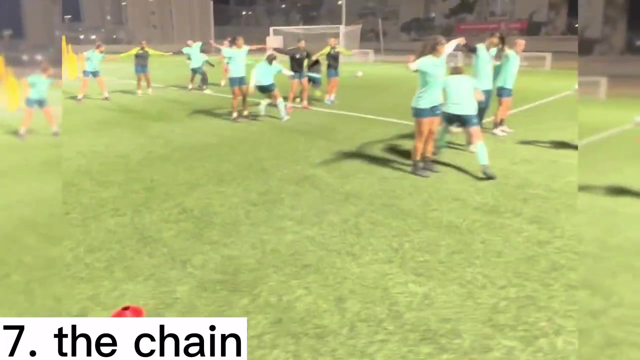 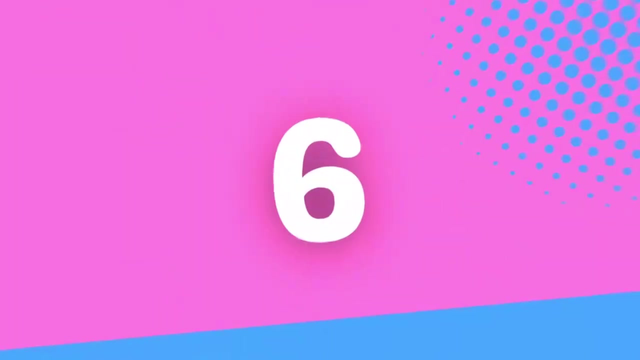 Go, Go, Go. Who scored? go, go, go. yes, yes, It's too late, You're too fast. Where's the balloon? Shoot, shoot, shoot, shoot. Aaaaahhhhh. Come on, get up, get up, get up. 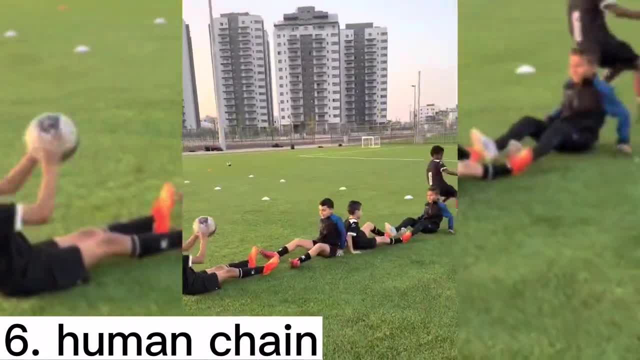 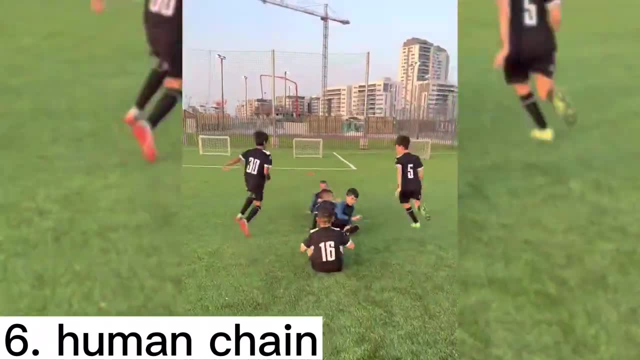 Good, come on exactly. active cooperation, Keep going. good, Nice, Go on, give him a shot, give him one, Go on, give him one. Move, Move Nice, Nice, Keep moving Nice. here's a good one. 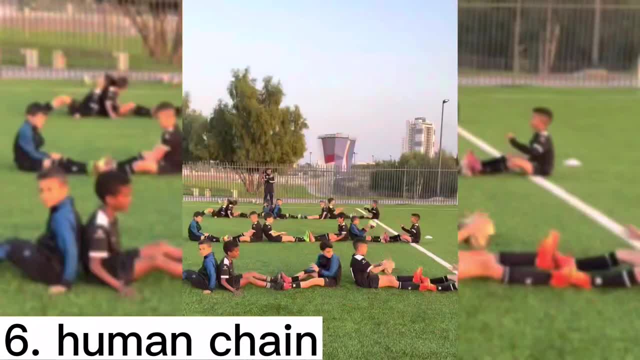 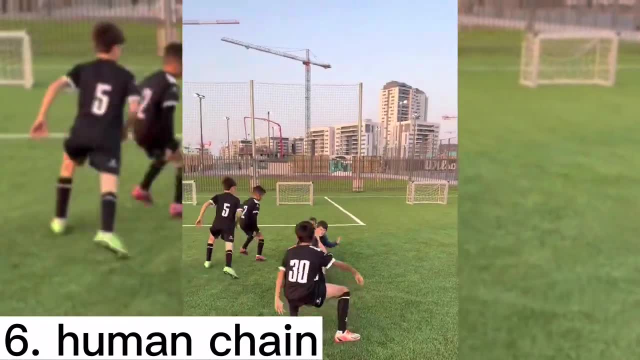 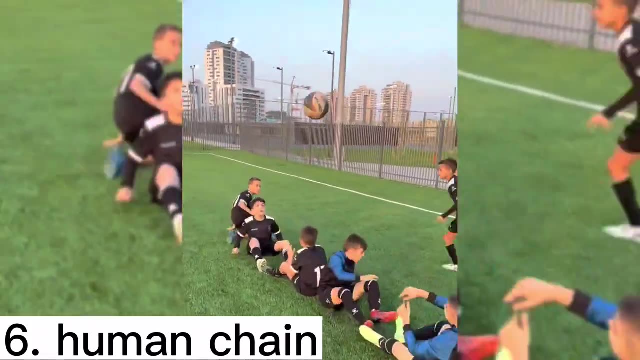 Good, Come on, you can move. who's going to jump? Who Move to the side? Yes, stop stop Two. good, You can come with me. You can come with me. Move, move, move, Come on, move, move, Come on, move, move. 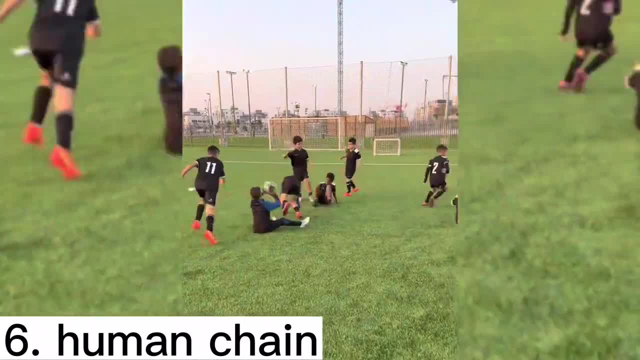 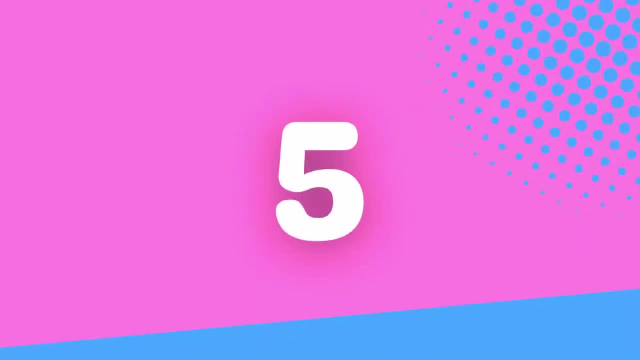 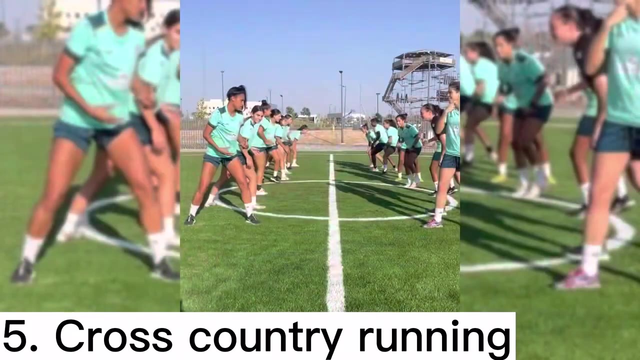 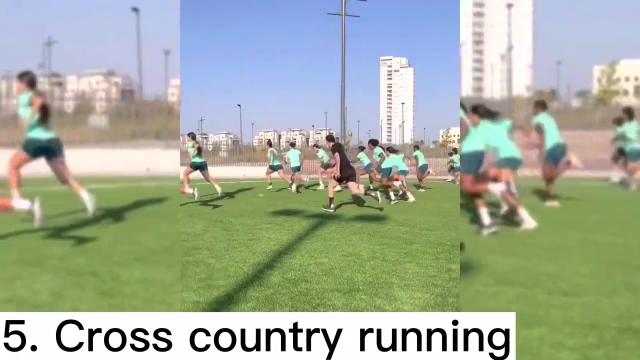 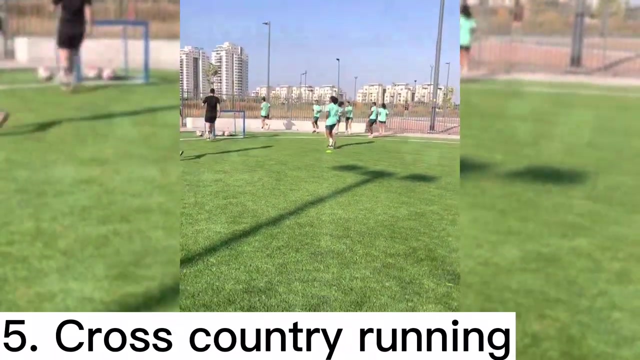 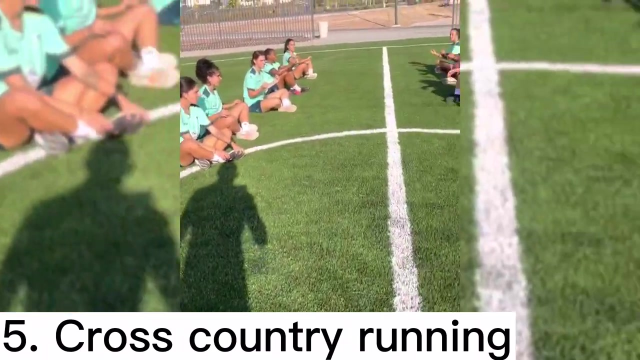 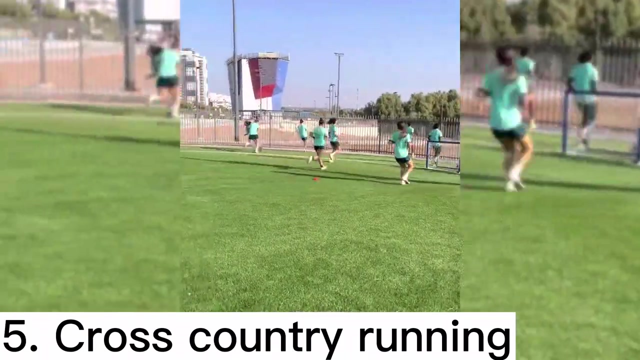 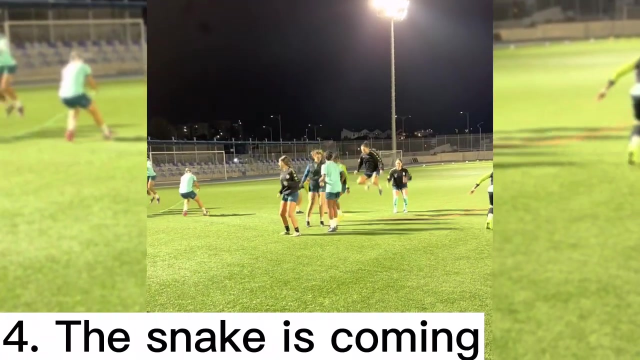 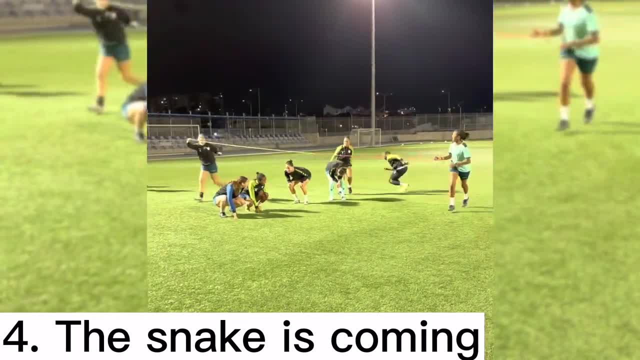 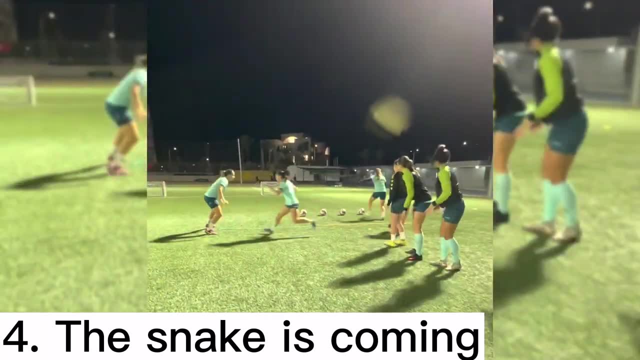 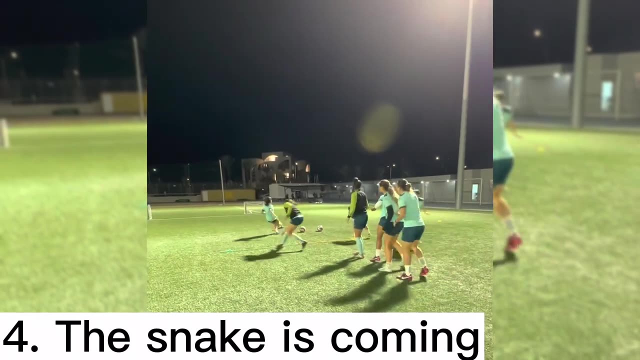 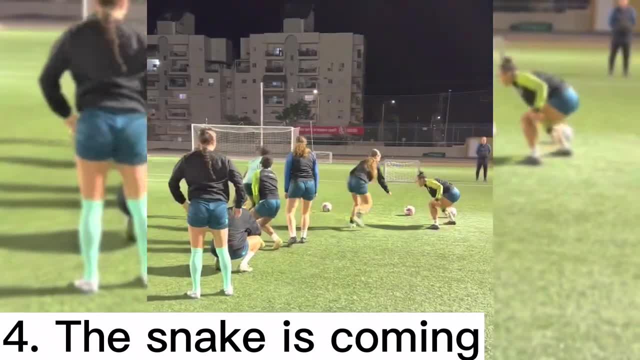 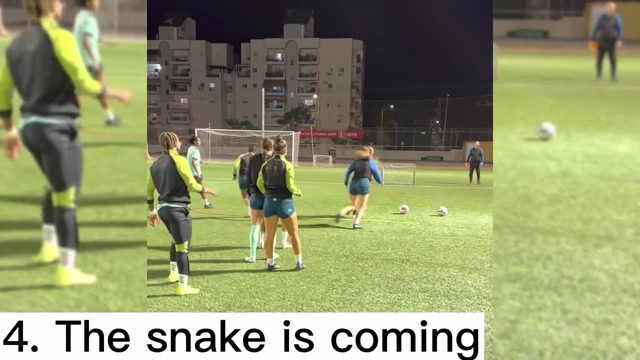 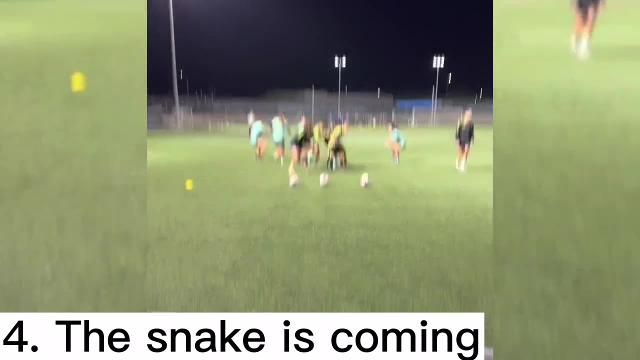 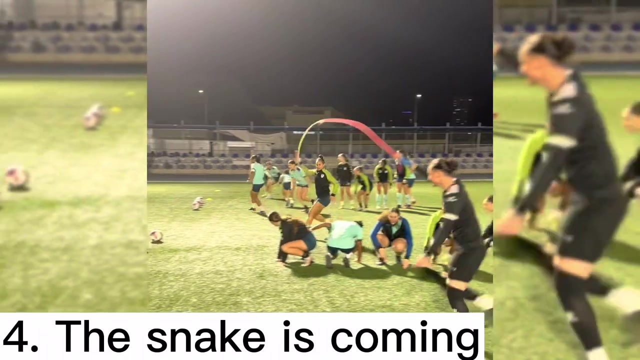 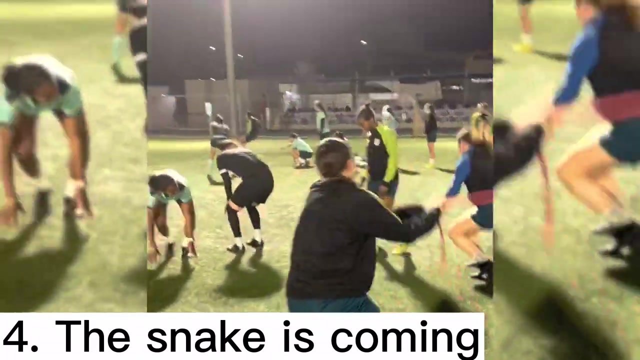 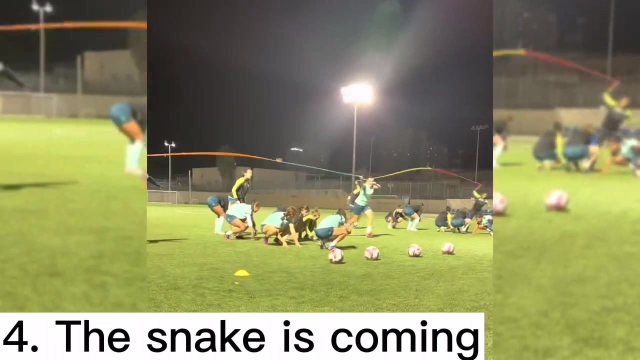 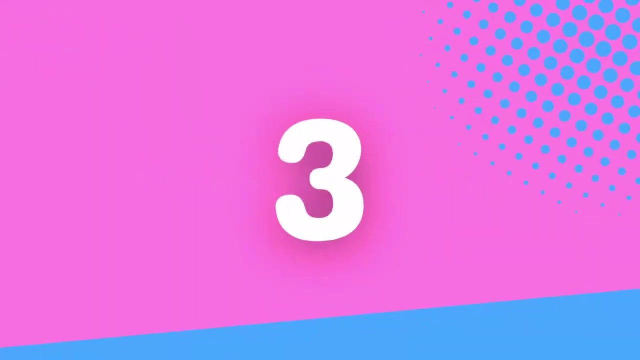 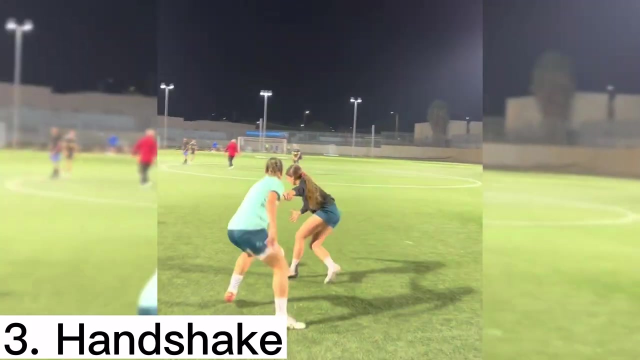 We've got a popping machine, Phobobopopop. Shoot, shoot, Go one outside, Kill him. He escaped 아니. Oi, Oi One, Yeah, Yeah, Yeah, Yeah, One one, Yes, Yes, Yes, Yes. 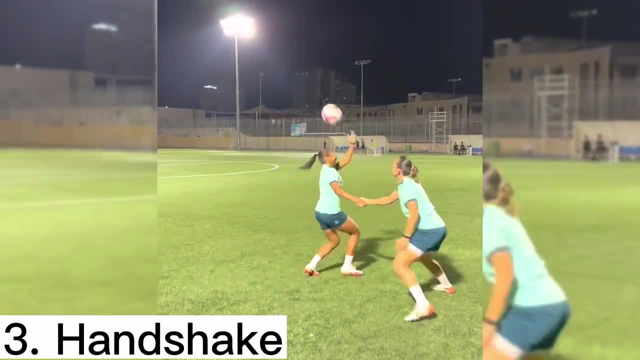 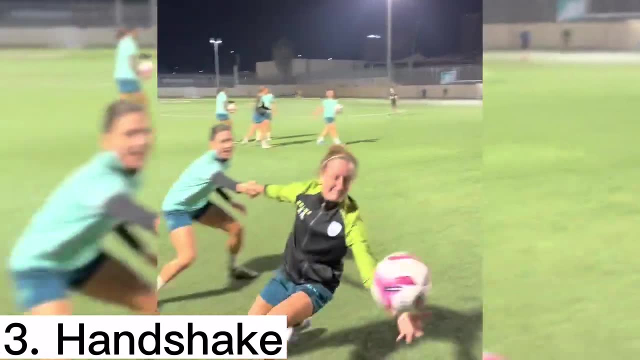 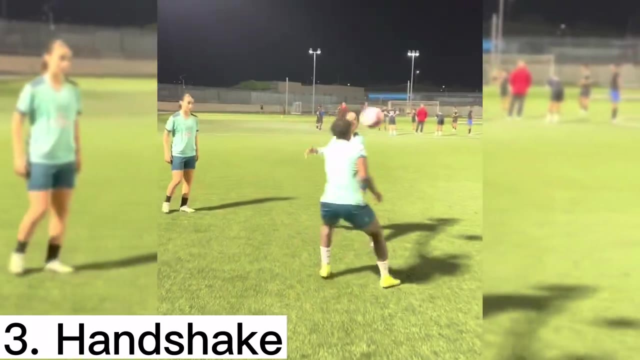 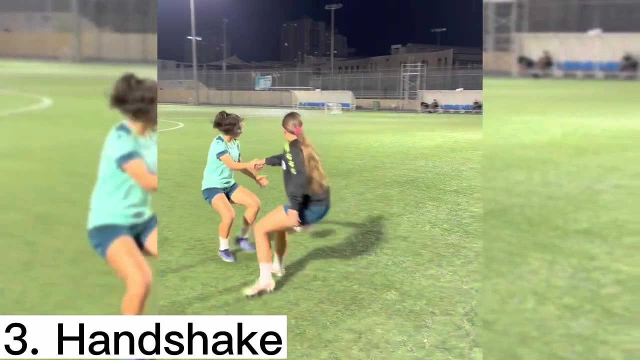 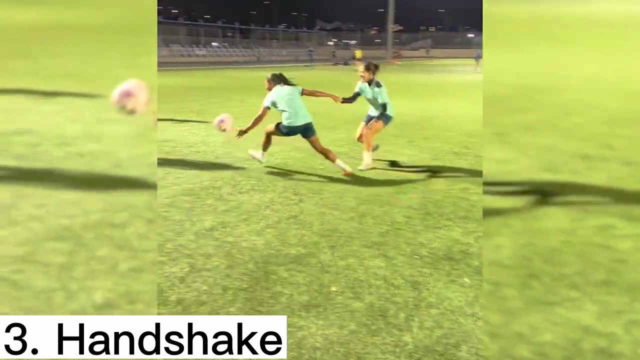 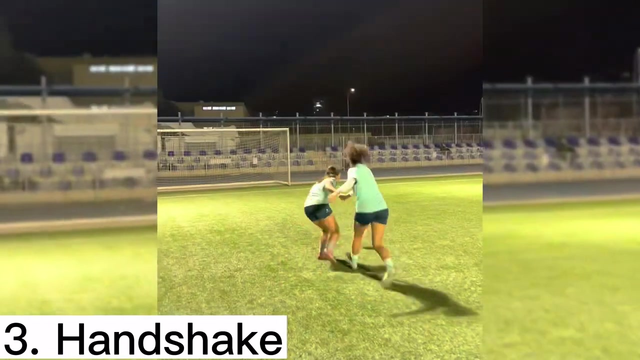 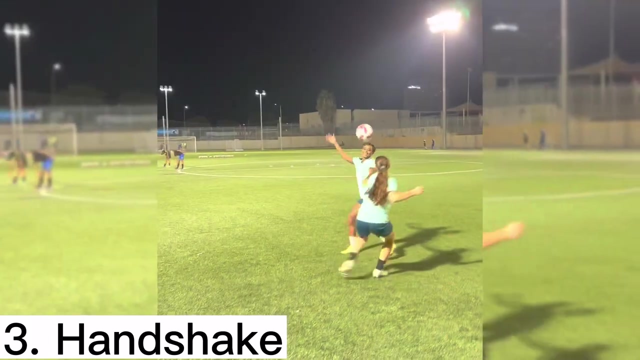 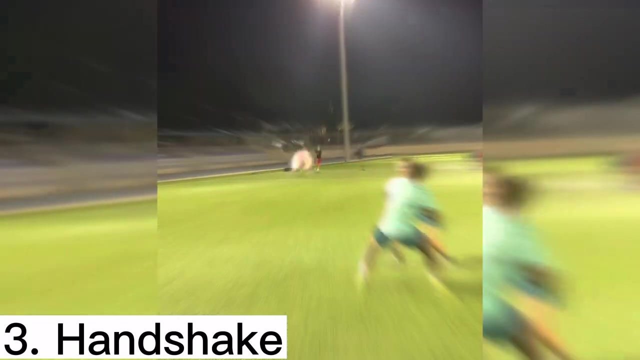 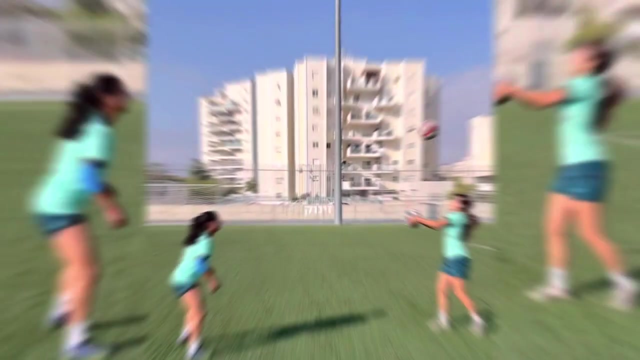 Yes, Yes, Yes. I don't understand why, I don't know. Hey point to Nikol: Nikol in front, Are you ready? That's nice, Good, Good job Killing. Okay, Benzaker, you have to survive. You have to survive, Good Wait. 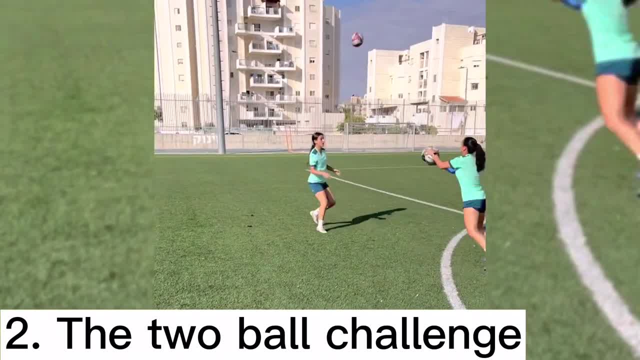 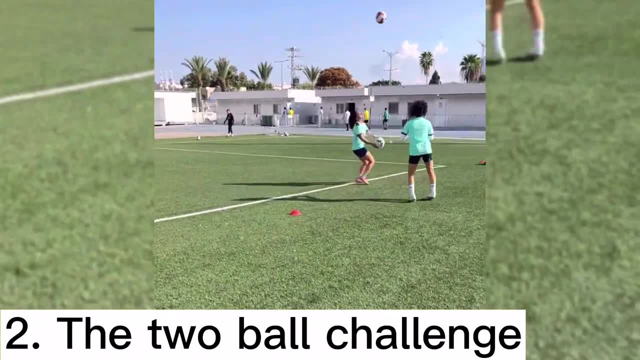 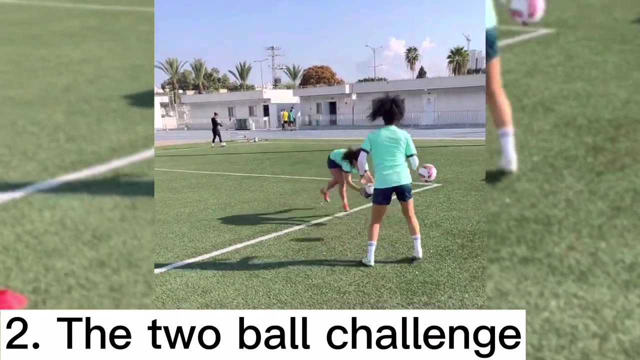 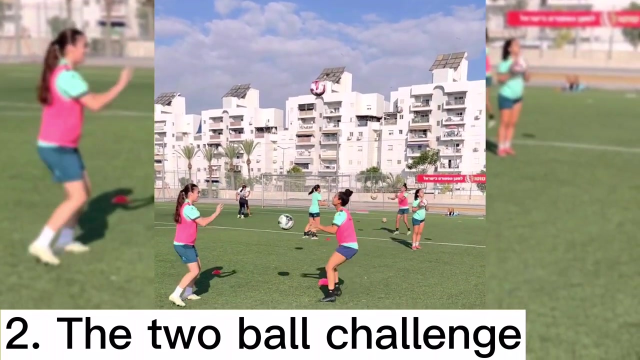 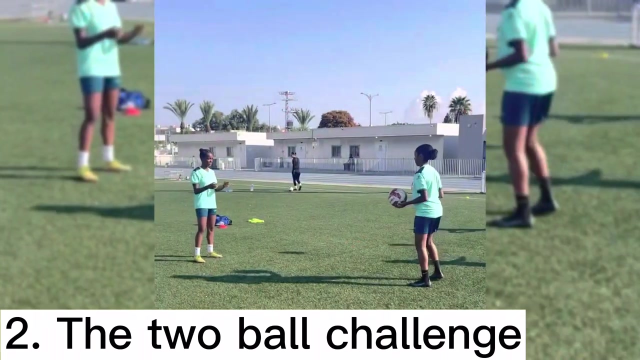 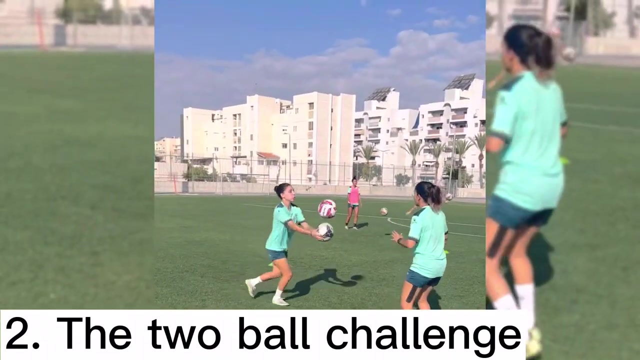 Good, Good, Come on. good. One more Here. it's good, it's good. Here we caught. Finally we woke up. Higher, Good Batul, Good Batul, What a control Batul. Good, Great, Killing, Killing. It was five, There were five. I want to see. 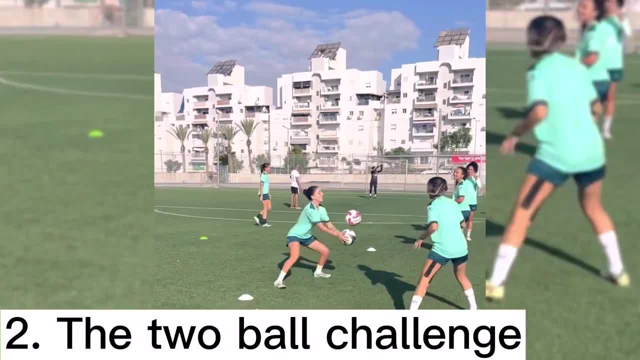 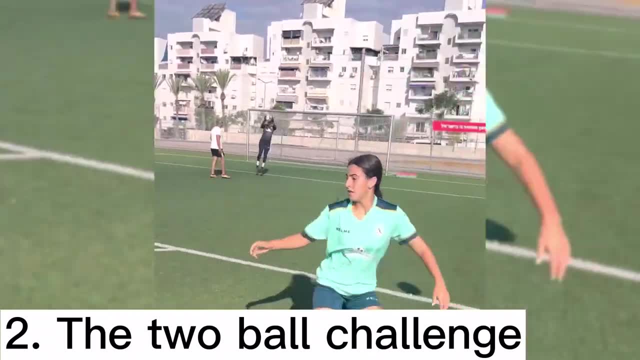 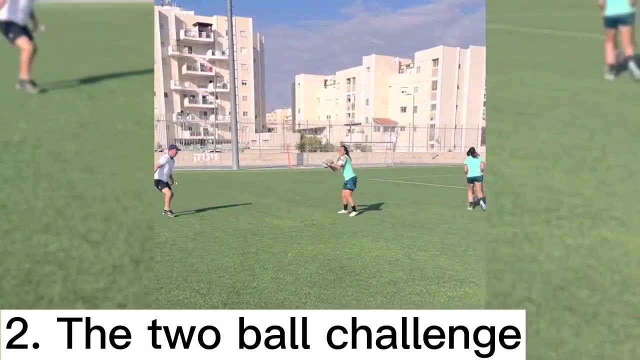 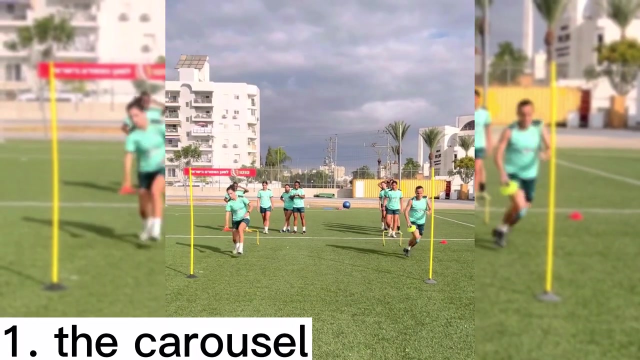 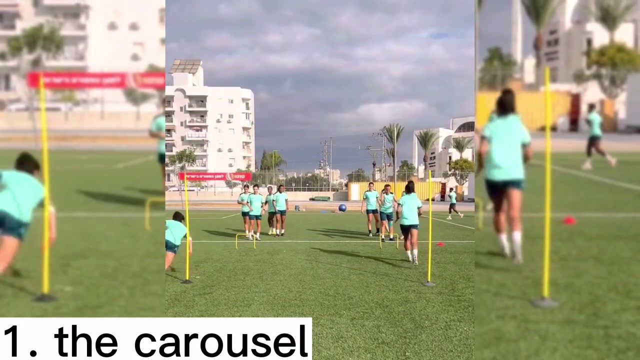 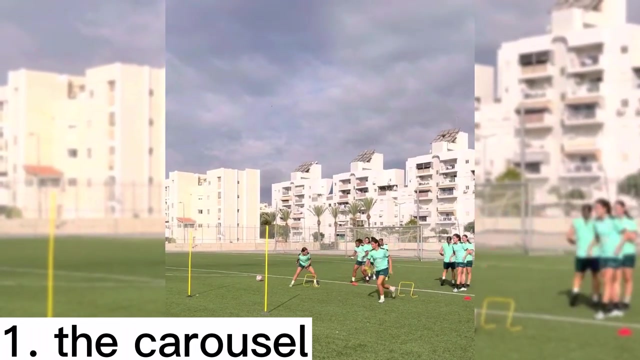 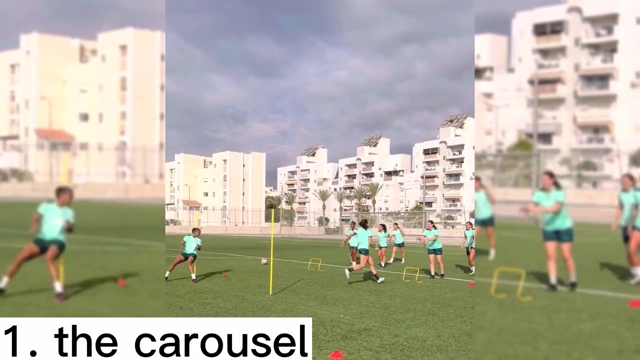 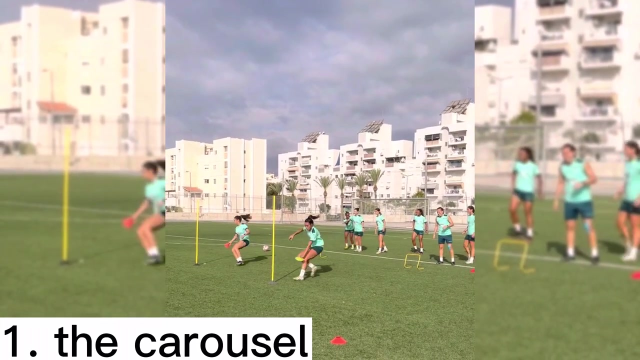 Killing, Killing, Killing, Good, Killing, Killing. Bring me Go go, Big guy, Come on, Good, Good, Here we caught Killing. Give it to him. Go up Longer. I La face. No, it's me No, but I Last one, Ili Ili. 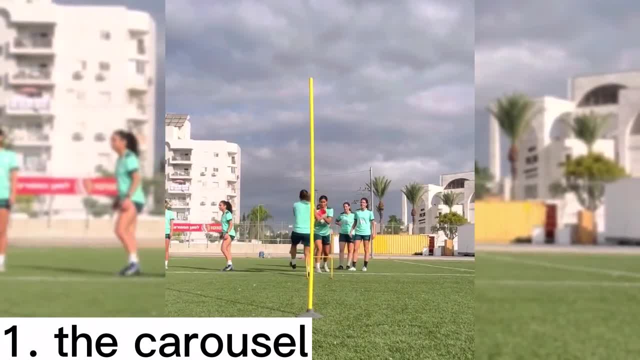 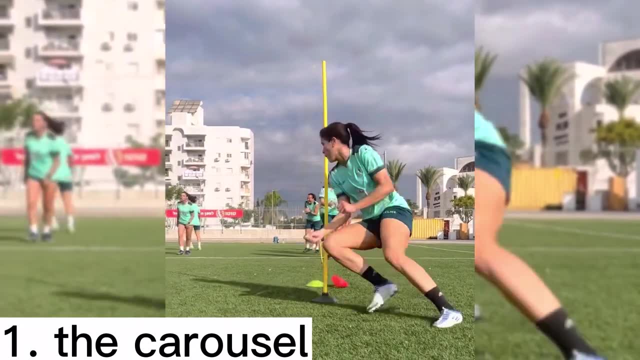 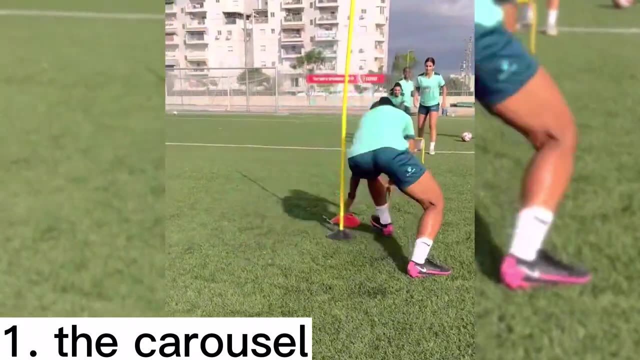 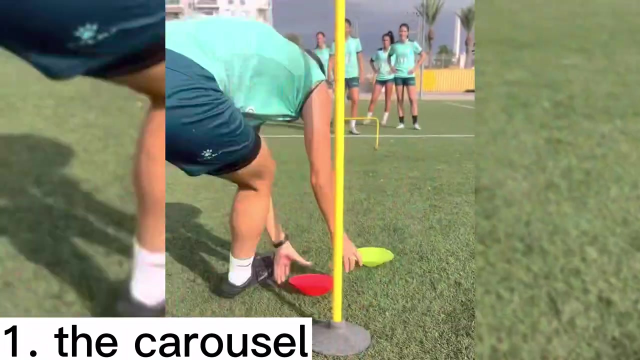 Come on Liv. Come on Doda. Come on Doda. Come on Shach. Come on Shach. Come on Shach. Okay, Shach with a break. good, Okay, Thanks for watching.